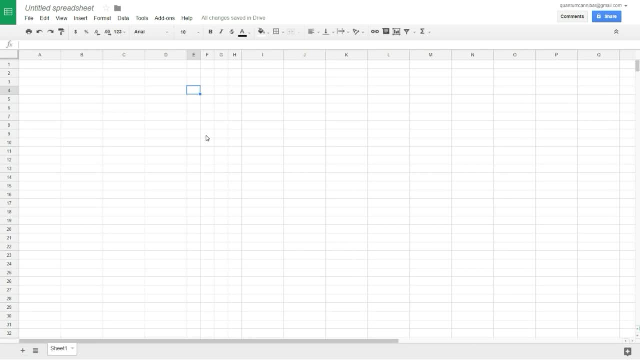 So in the first example I just want to illustrate the sort of key behind the squares. You just got to make sure that, like Sudoku, that they are sort of unique In the way that they're created. So let's just do 1,, 2,, 3, 4, and then 1,, 2,, 3, 4.. 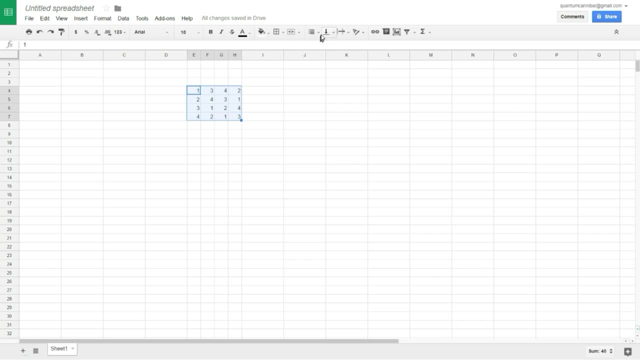 Now, this is a really basic sort of square, Just to, like I said, just to illustrate the reason for the uniqueness. Okay, Add that up And I'm going to build off this and I'll build a square just like the one shown in the Tengri. 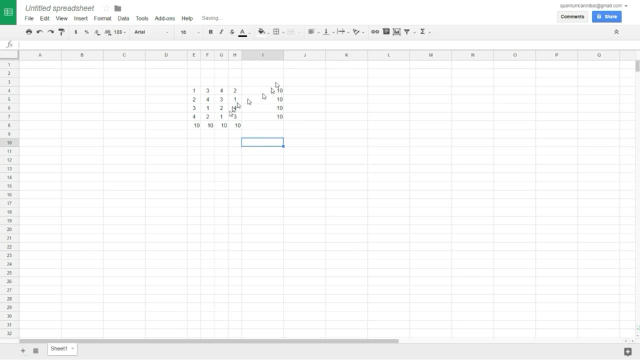 puzzle, But I wanted to show you this first. See Now logically, yeah, So 1,, 2,, 3,, 4.. Add those up, You get 10. And of course, the same way over here. 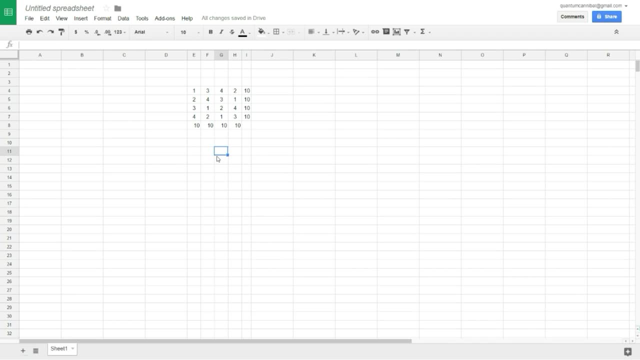 Same way over here. Same way over here, Okay, But with the Tengri stuff it's, you know, they don't have just four numbers, They have 16.. So in order for me to do that, what I need to do is create a second set. 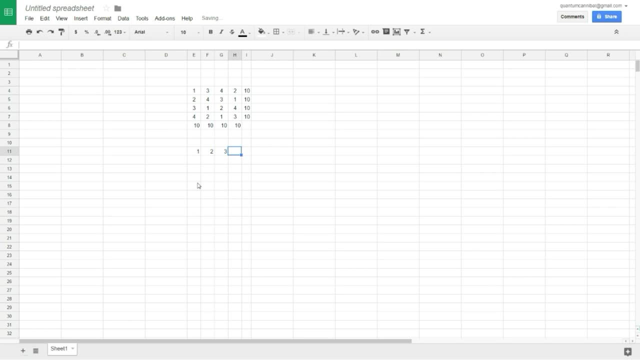 So let's just do you know 1,, 2,, 3,, 4. Or 4. Oh, is it 1?? So what's like you can't Actually hold on. Let me do it this way. 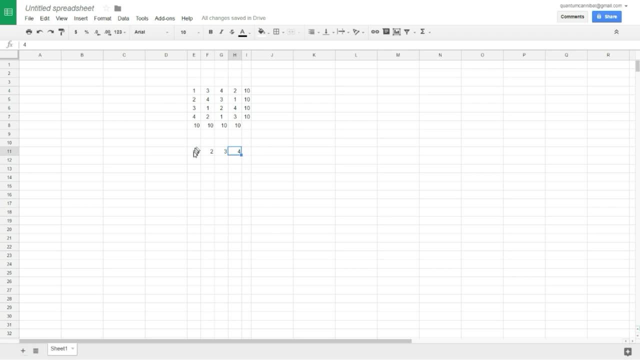 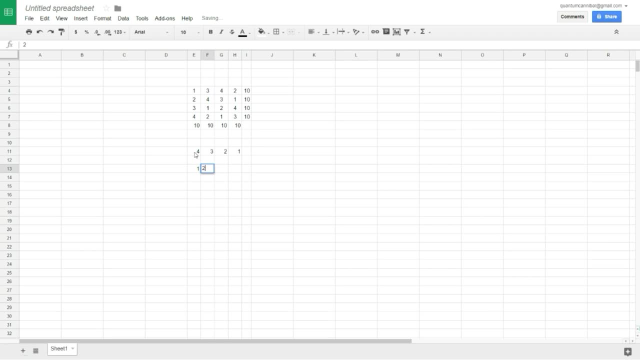 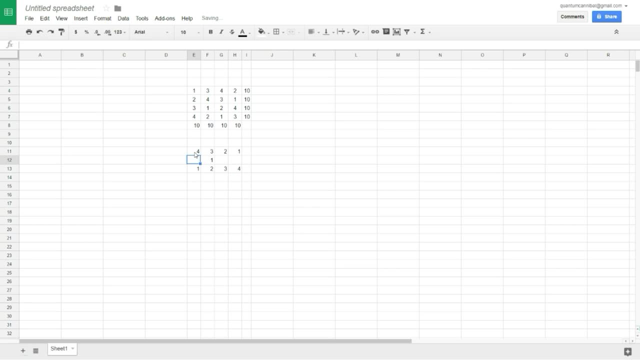 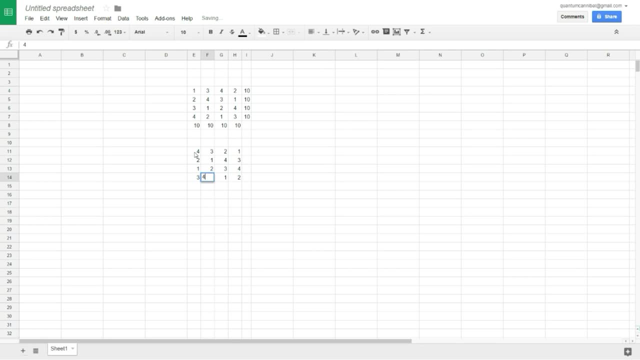 So now we have another unique square. I just really I just turned this one on its side And what I'm going to do is I'm going to take the number from here and the number from here and combine them to get another set of numbers. 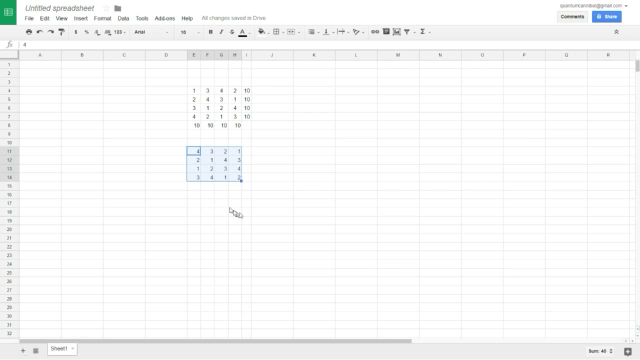 So it would be like 1, 1, 4.. 1, 2, 3, 4.. 1, 2,, 3, 4.. 1, 2,, 3, 4.. 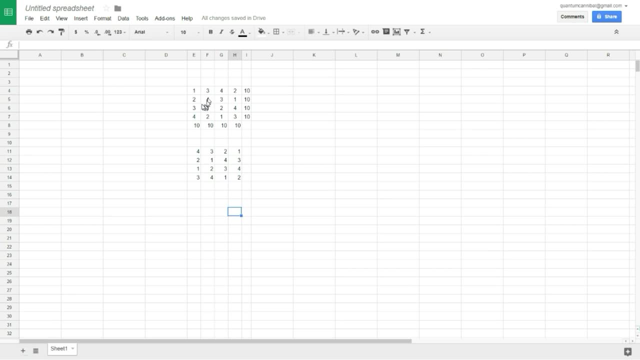 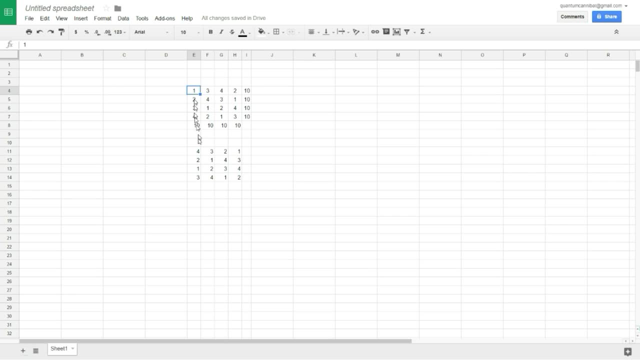 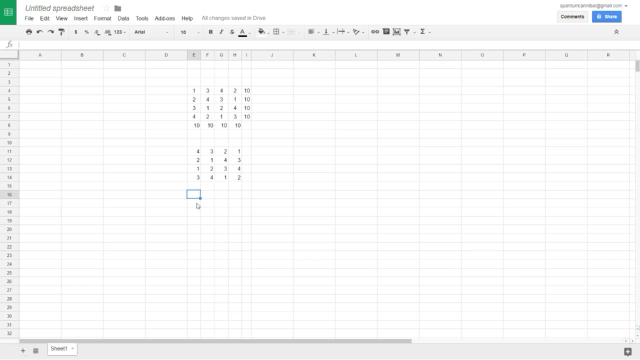 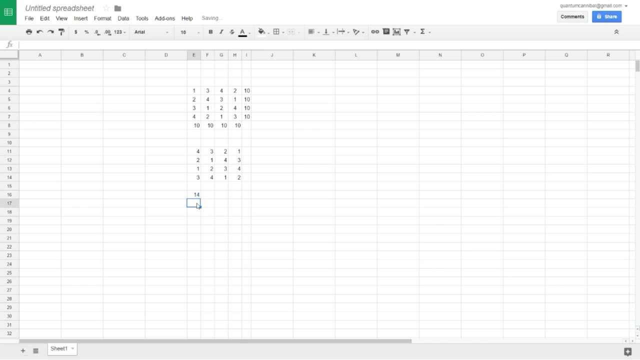 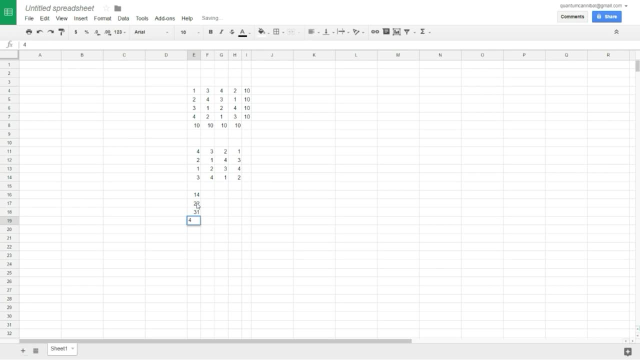 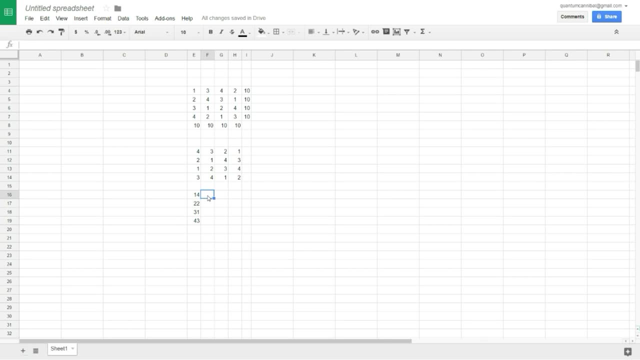 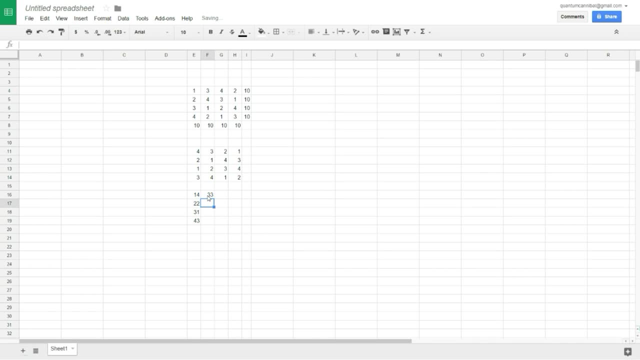 But I'm just sort of showing you so you understand what I'm doing here. I'm just getting a unique set of numbers: Two, four, Two, four, three. one, two, one, two, three, four And three, two. 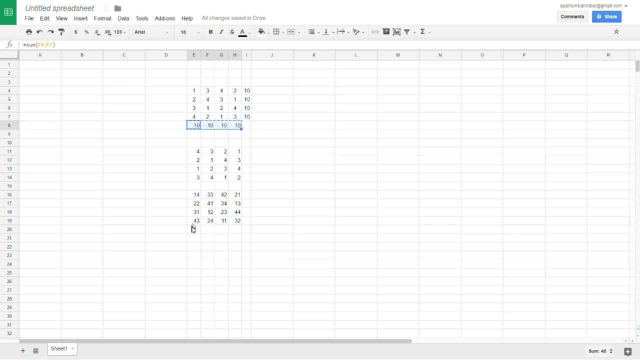 So now, if I add these up, I should get another, another, yeah, okay, another square, Okay, so that this is our sort of framework right here for rebuilding the Tengri stuff. So what I'm gonna do to sort of help. 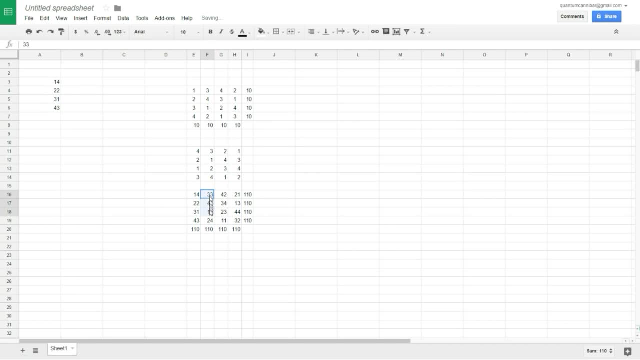 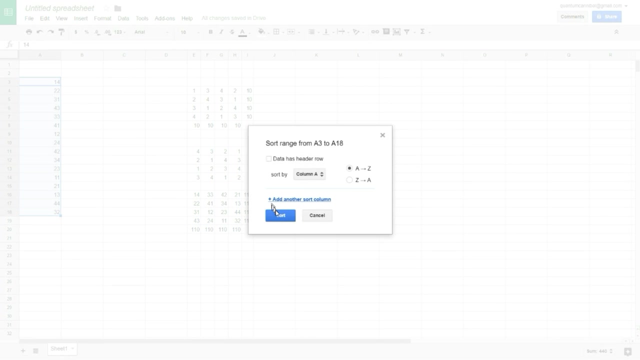 with generating new ones is. I'm gonna copy all of these numbers so that we have a reference and a simple calculation to do it. So let's sort these, sort this range, And now I'm gonna just show you something interesting about the range. 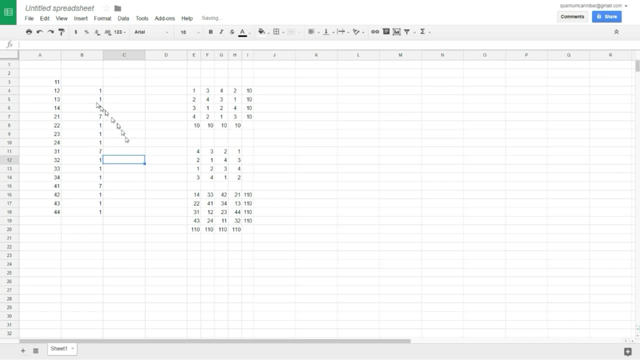 So these numbers are important. here, You'll notice, was sevens, sevens. I get to mess with those numbers, So let me just repeat or recreate that formula. So this is one plus this, And that's really all. it is going all the way down. 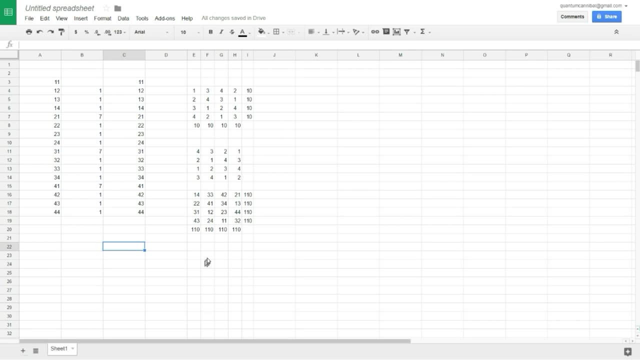 Right, so we got those. Okay. now the next step is to sort of recreate this square, but using- yeah, just Angela, and then either Sage these numbers as a reference, so, and i'll like, i'll fast forward it so you don't have to watch. 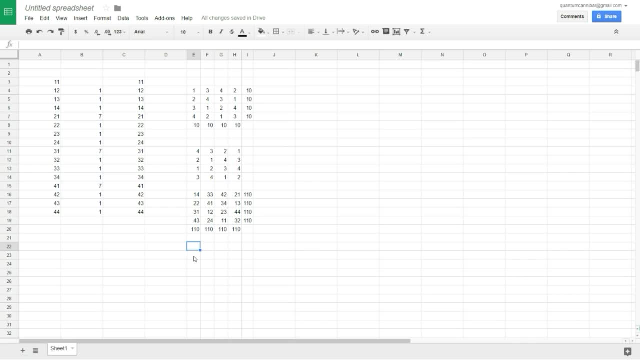 me go through this, but i'll. i'll show you the first row. i basically got to do the same thing for each row. so this one's going to be 14, so 14 is here. this one's going to be 22 and 31, 43, okay, and then i just do the same thing for the next three rows. 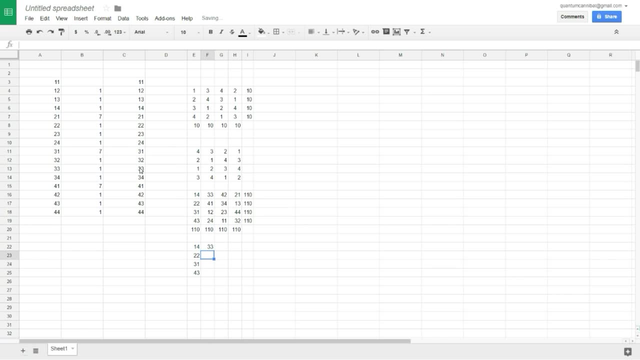 and through the power of video, i'll fast forward this so you don't have to watch it. so okay, so now we've recreated this up here and, of course, if i just um do the calculations again, um, we'll get the 110. so now what i have here, um. 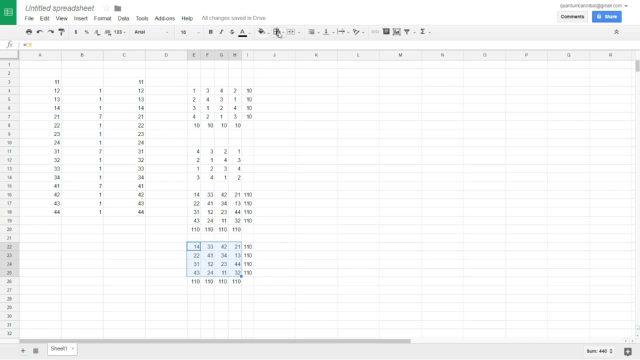 is this magic square that now we, we can now play with by changing these numbers up here. now the ones you should kind of focus on, are these, these, these four values here, um, as they change. so if i change this, i'm sorry, it's this, this, this and this is what. 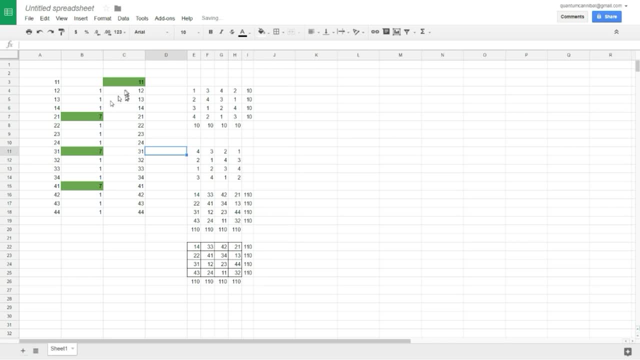 you can change um. so from here, say, i do 23, um seven, three. sure they don't have to be primes, i'm used to using primes- um you'll notice that all these numbers are changing, and so is the value of all the magic squares. now, if you follow, if you follow along, 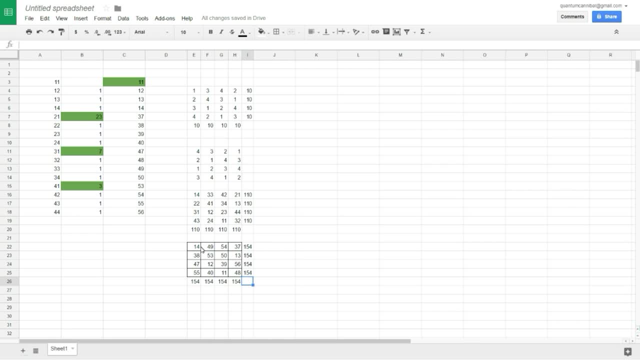 um, it's, it's just the uniqueness of each one of these values. um, using this simple formula here, i mean i could change these to one, you know, and i'm still going to get a magic square here now i guess really, what uh tengri wants to do is to change these to one. 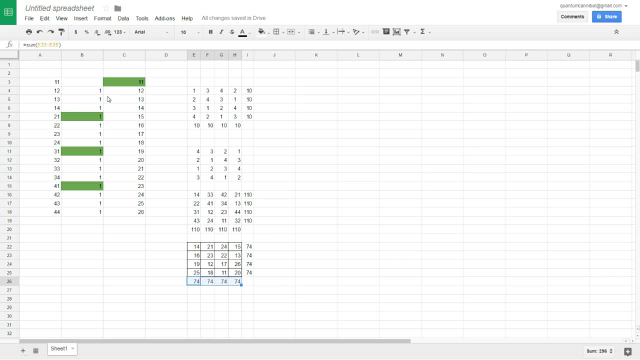 three seven. so we're going to give him a sliver here and we're going to program this, and then we're going to program this thing to a number plus one, to one uh, zero, so that he can. i'm going to do one three seven. then let's go to the original number. one. one three seven did was mess with the. 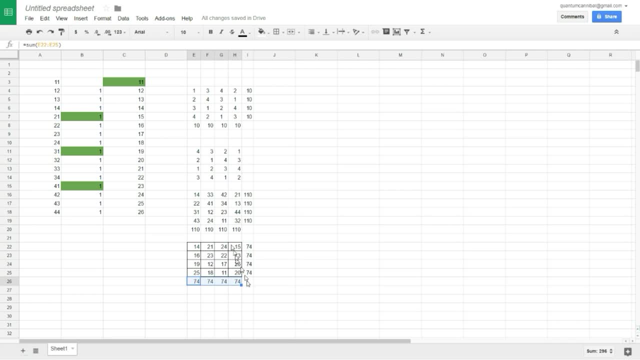 numbers enough so that he was able to get um six, six, six for all of them. so let's do do a seven, seven, seven, seven, um. uh, let's see if we can go 17, let's do 150.. 168.207.106.257,000.470.839.8351.936. Olivia said we are going to do 60-70 this afternoon. 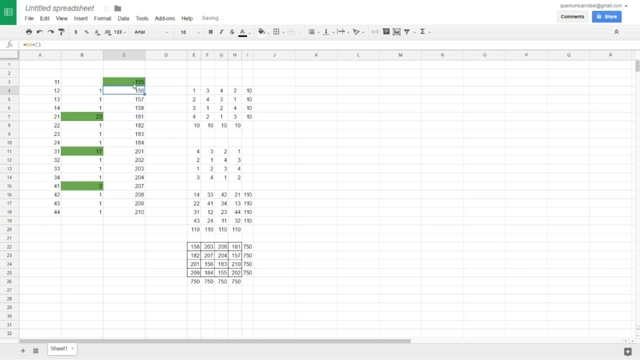 oh, you know what? I'm never gonna get it this way. these are all even so. you kind of play with these numbers a bit until you get an odd, like that. so you have an odd number. there you go. so we have our own sort of seven, seven, seven, magic. 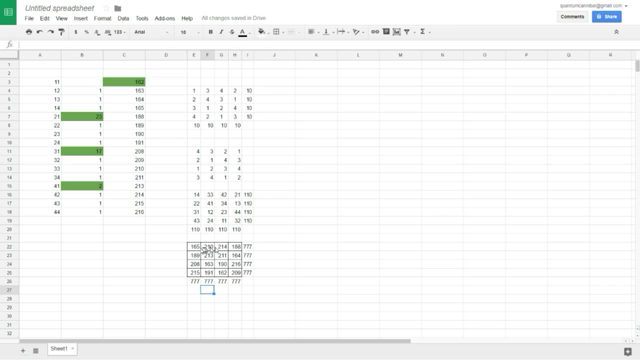 square. now, that's one square. the other one had multiple squares. I don't recall how many were, maybe six, eight of them, but that's just another trick using the same square, and the way that you can do that is, essentially, whatever you add to this one, you add the opposite to this one, then you add this one and 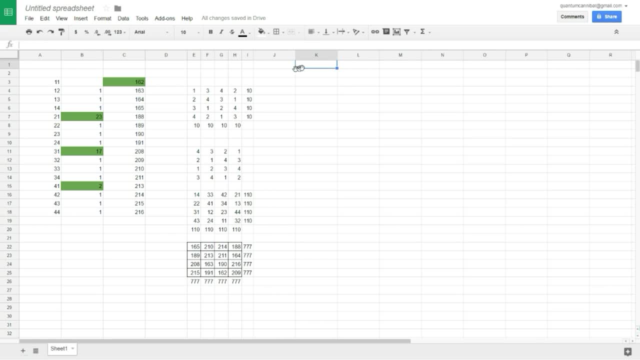 add the opposite to this one of the same number. I'll show you how that works. so we'll just take number two, because I'll need that, and I'll say 2,, 2 times this value, times negative one. so we get negative 4 and I'll. 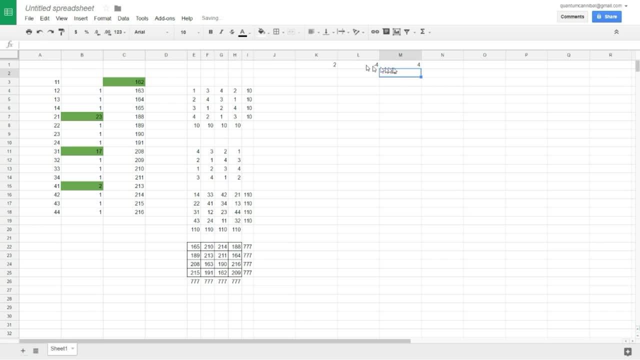 we'll do this times negative 1. I'm only doing this so I don't have to do it manually for the square, oh sorry. and then again it's: it equals this times negative 1, and then these again, and you'll get this kind of flip flop. 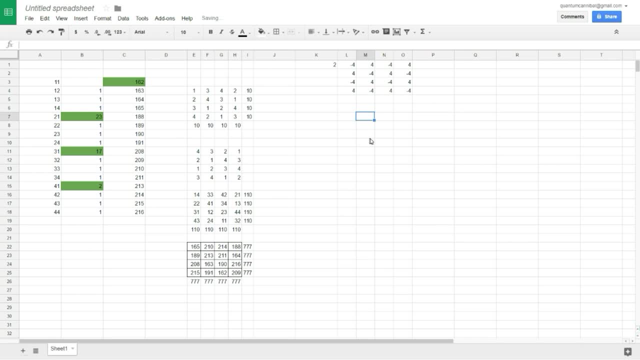 like this: minus 4, 4,, 4, 4. ok, and then what you do is you take this value, you add this value and we want to keep. so we have 161, 162, 163. so we just kind of paste this all down. 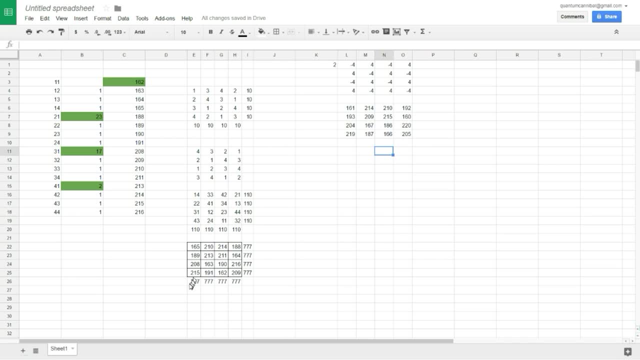 the row, we get an entirely different set of numbers, but because the map is pretty straight forward, you see, I'm taking 4 away from this one, but then I'm just replacing it on top of this one, and that's why you're getting the same number again. 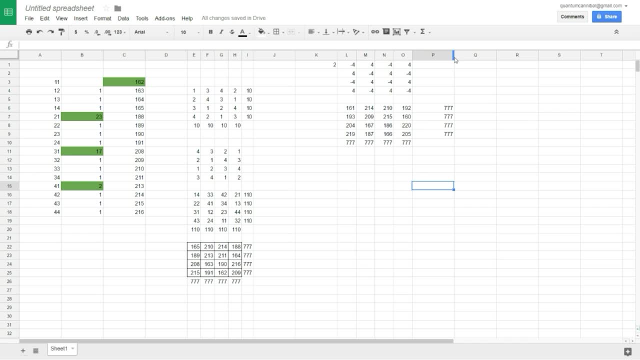 if you look at the Odin number, if you look at Odin's triple horn puzzle, and take one of the squares and then you take another square and you get the difference between the numbers. it's the same thing. he's just, you know, doing the math, so you can do this. 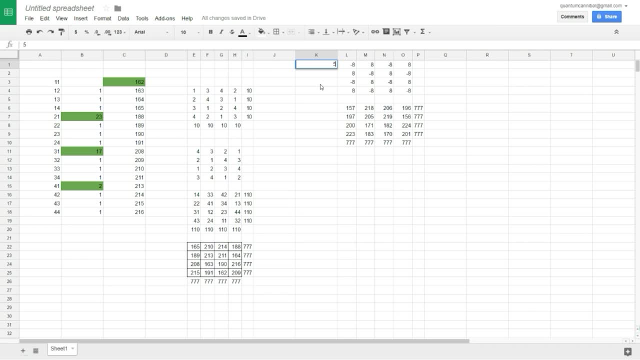 so let's do 4, 8, see how they're all. they're all different numbers, they all come up to the same value. so that's it. um, just think about it, just think about it, just think about it. just thought you would be interested in seeing how the